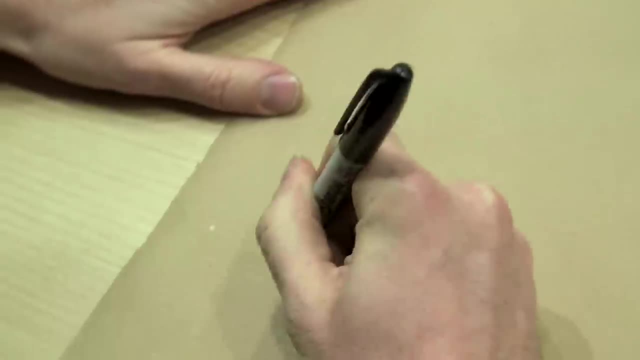 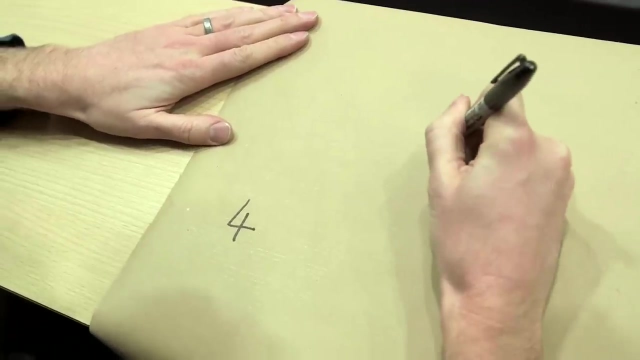 Okay, right, so 42,, 42,, 42,, 40.. That gets smaller, 2.. Alright, there's more. I'm just I'm starting with those digits. I'm gonna put a 5 in over there. 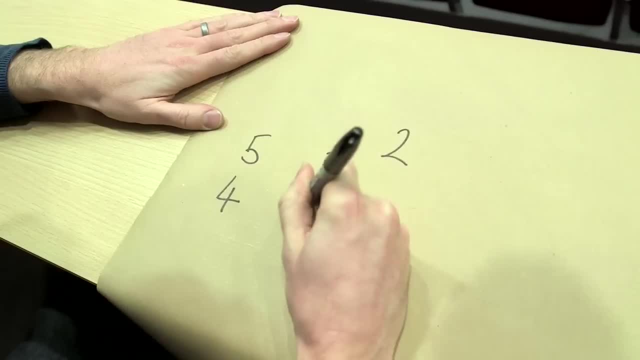 I'm gonna put a 3,. actually I put a 3 there and a 6 there. I'm allowed to change it as I go. That's gonna be a 9,. that's gonna be a 10,, a 2,. 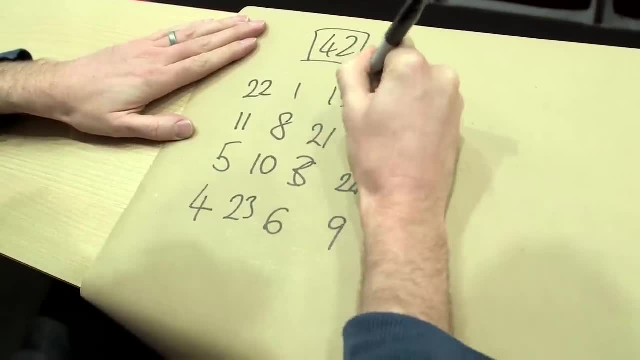 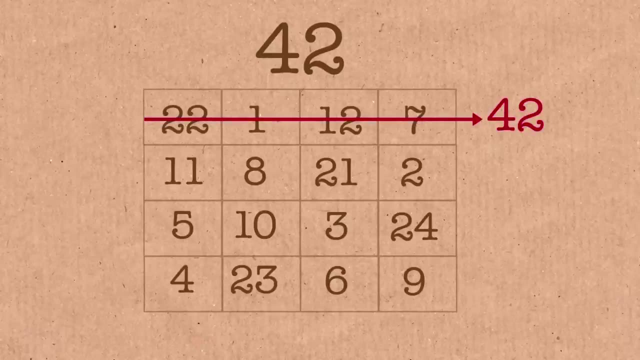 23,, 24, and 12.. And what I've done for you there. if you double-check, all the numbers in the top row will add up to 42,. if you go through and check those, The second row will add up to 42, and all the columns up to 42,. the 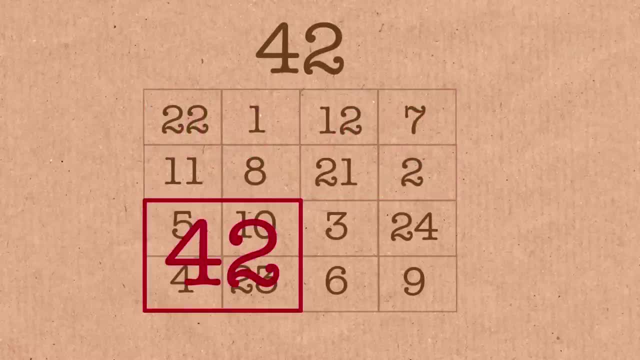 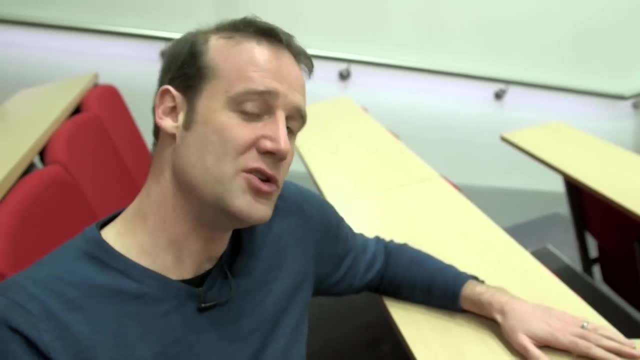 diagonals are 42, the opposite, I mean all four in the corners up to 42, each four in the corner adds: it's a magic square. I love magic squares, mathematicians love these a lot. and so there that. that for you, Brady. 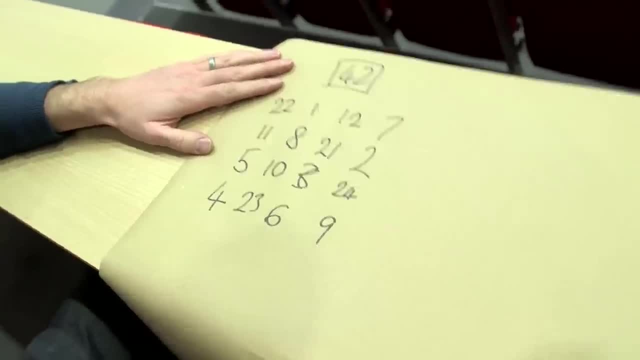 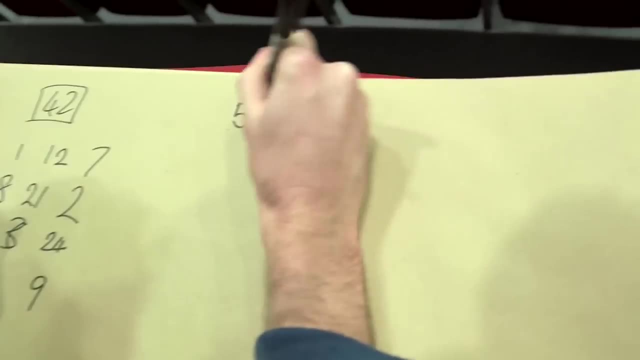 that is. that is a gift magic square based on number 42.. Now make one for 58.. Look at him, think 50,. okay, let's do another one for 58.. This one's gonna be wildly different at 58.. 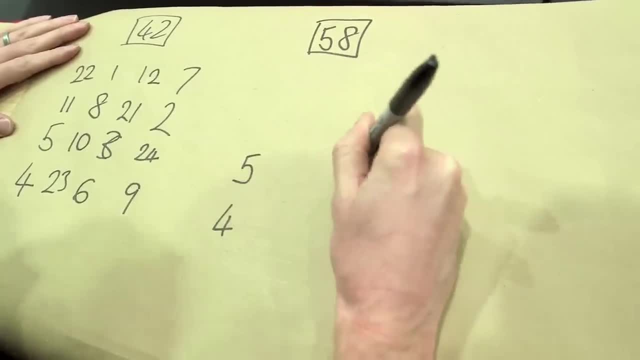 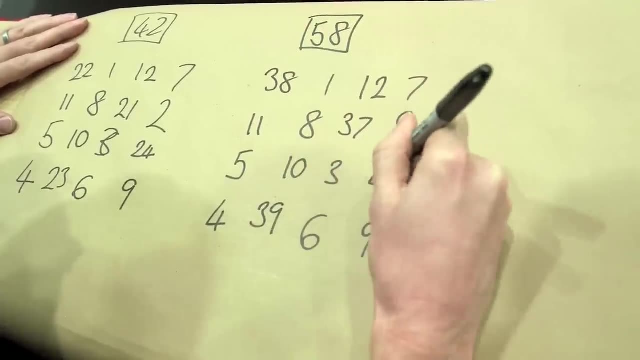 So I'm gonna put a 5 there, I'm gonna put a 4 there, I'm gonna put a 3 there, I'm gonna put a 6 there, I'm gonna put a 1 there, 8, and then that one's 38, and then 39, and then. 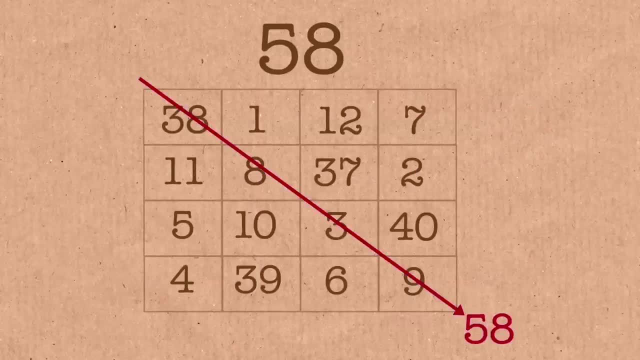 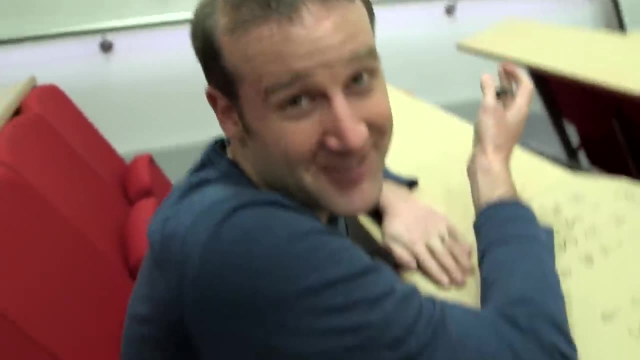 40, and there you are: An incredible amount of mental arithmetic. later I have managed to you look unimpressed, I'm gonna be honest. uh, so I am. I am, yeah, the first time I was impressed. now I think maybe you're just using a proforma in slow motion. 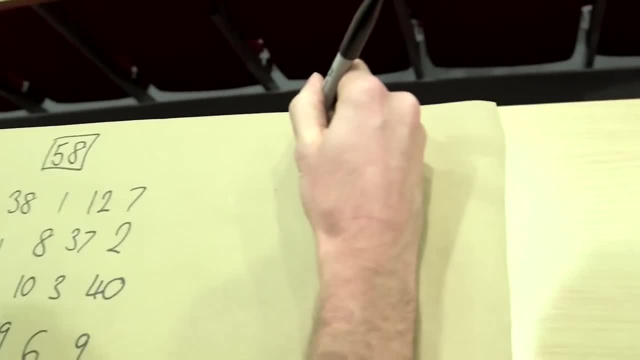 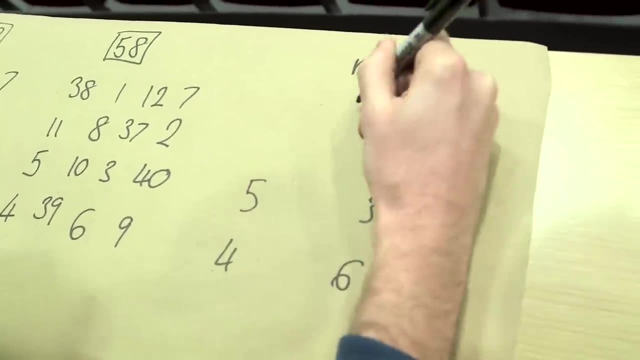 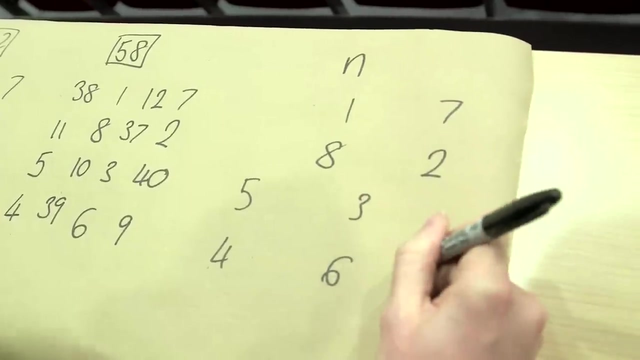 Maybe. maybe all I'm doing is, if you gave me the number N, then I'm going through and I'm doing: these are all exactly the same every single time and so I fill in those and these are easy to remember. these are the multiples of 9,, 54,, 36,, 18,, 72, then I remember I put 9 down there. 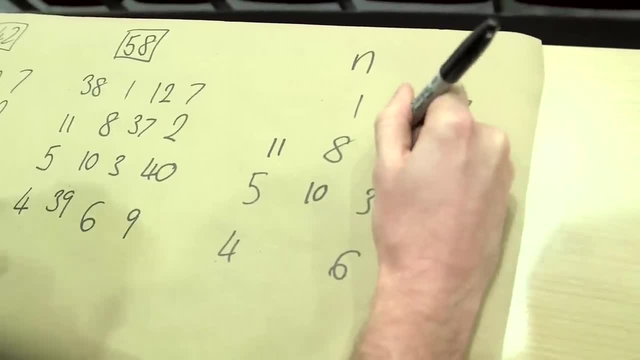 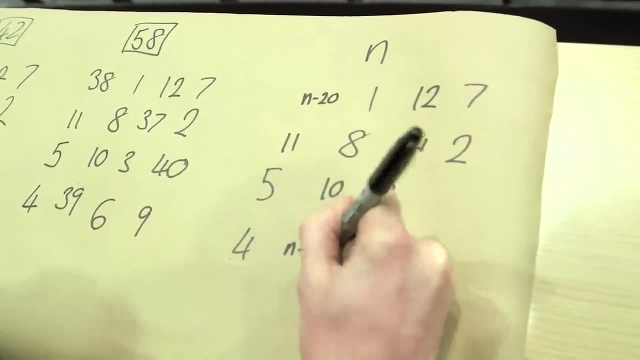 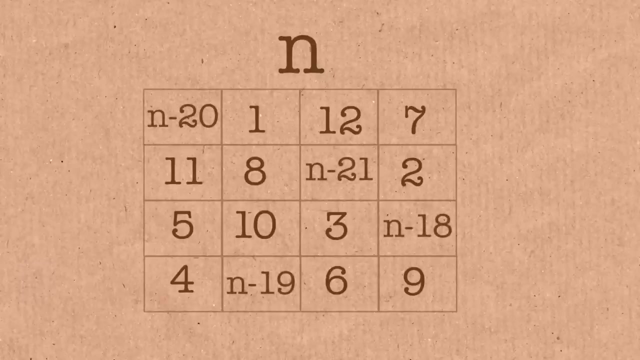 10,, 11,, 12,, and then I do N minus 21,, I do N minus 20,, I do N minus 19, and I do N minus 18,, and that is a magic square. The problem, of course, and the reason it gets a bit suspicious with big numbers, is you can look at this one here and you go. 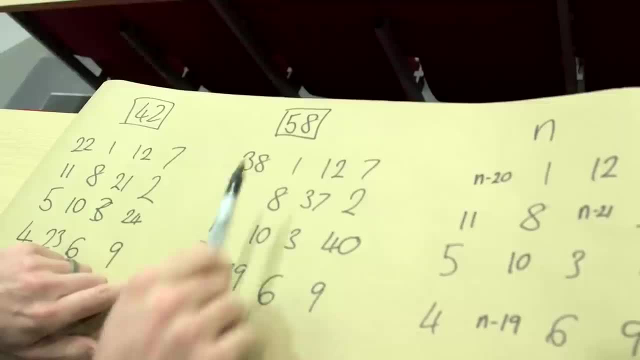 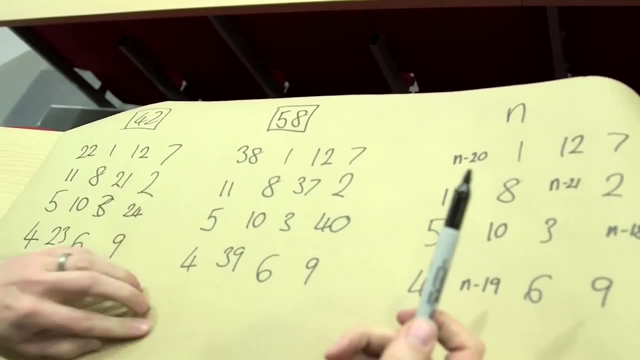 wait, they're all quite small. and then what's this? There's like suddenly some massive 30s and 40s going on. You'd be a little bit unimpressed. So even though you gave me 58 out of nowhere, you look at this and be a little bit suspicious. so 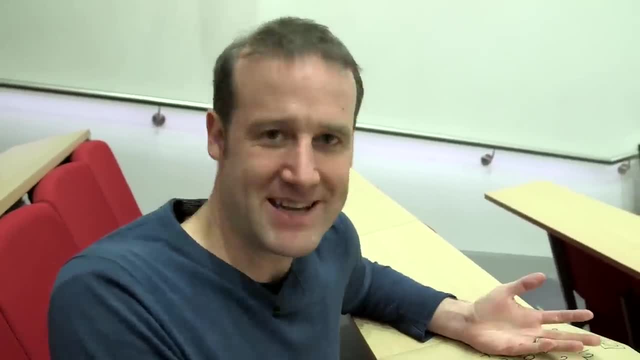 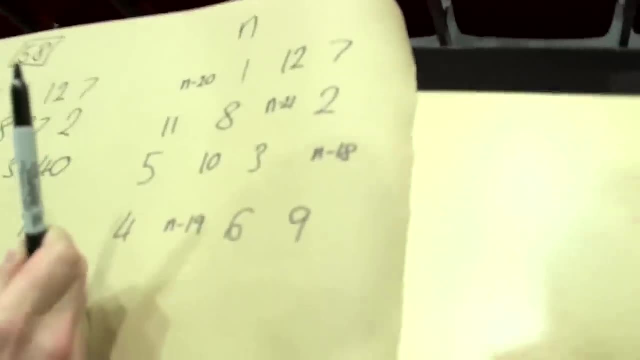 So that's why ages are often good. Ages are often good because they tend to be in around the 30s and 40s is perfect. Anything too big starts to go awry. There are- But what about small? What if they because-. 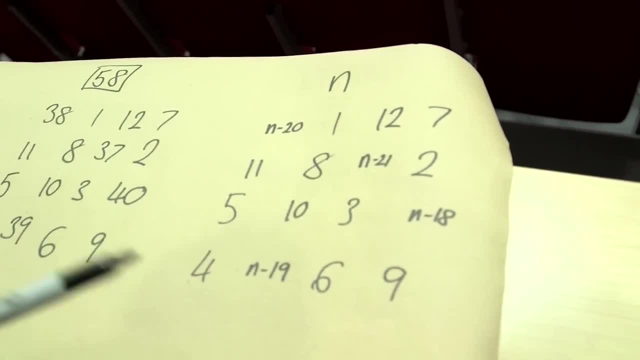 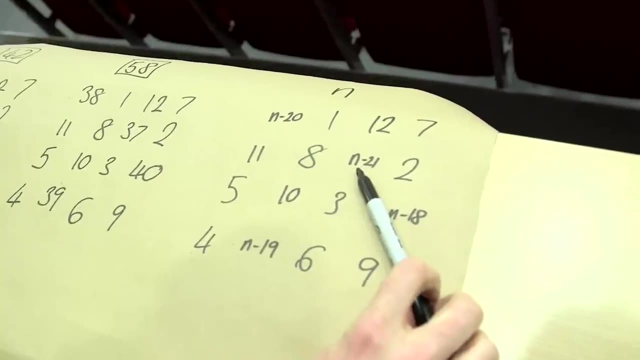 What if they give you like 8?? Actually it, no. that's why I said between 21.. So ages are very good, because then this one, if someone says 21,, you have a 0 there, which I'm kind of okay with. I don't mind 0s, it goes 0,, 1,, 2,, 3.. 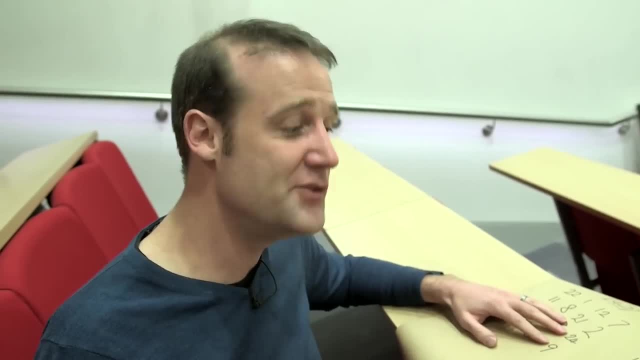 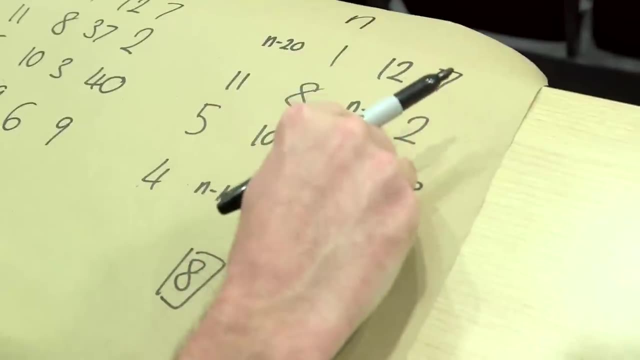 Anything smaller, you get negative numbers. So the square still works. if you gave me a tiny number, So if you gave me something like um 8, then I would have in that spot. there I'd have to subtract 21 off 8,. 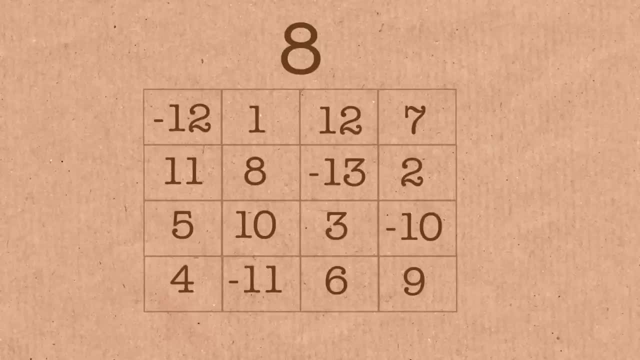 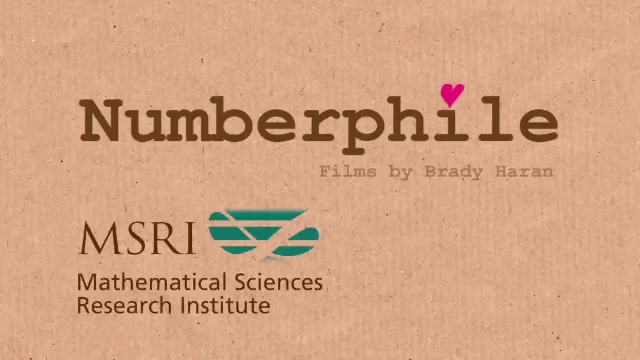 and I'd have a negative 13 hanging out in there. And if I gave you a million- And if you gave me a million- you'd have massive, massive numbers. All this diagonal, all that diagonal. they add up all this little square in here. they all add up to the same number.